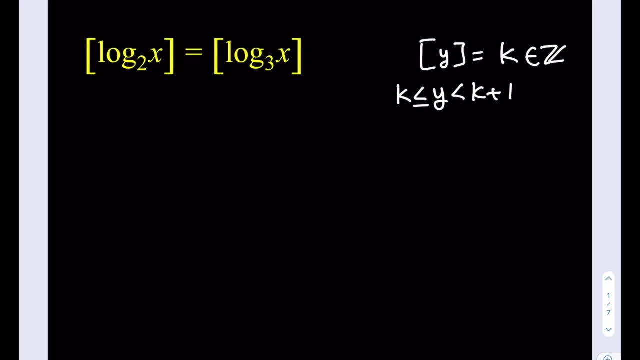 Okay, so that's basically how it's defined. So now, what we're going to do to solve this problem is: we're actually going to do the same thing here, So we're going to use substitution. Let's go ahead and set these equal to k. Now, what is this supposed to mean? Let's go ahead and each one. 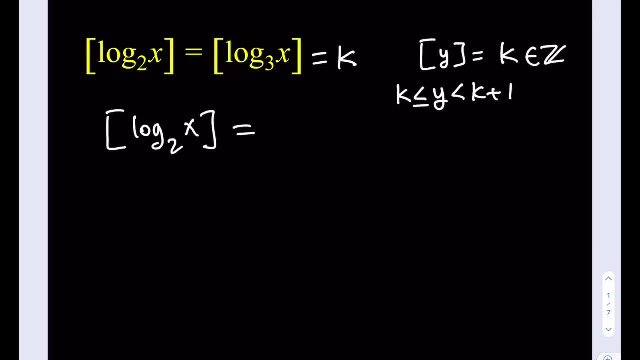 write each one separately. Log x with base 2 is equal to k. Now this means that log x with base 2 is between k and k plus 1.. So that's basically how it's defined. So now what we're going to do to. 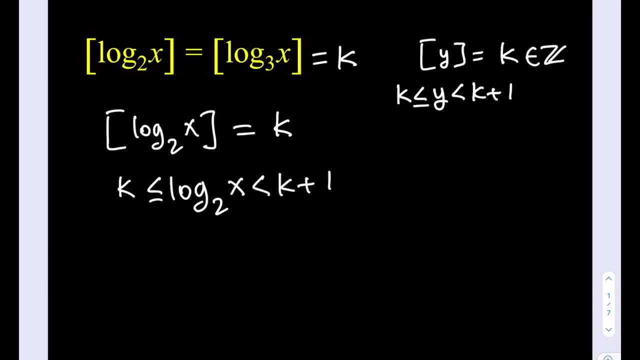 solve this problem is we're going to use substitution. Let's go ahead and set these equal to k and k plus 1, where k is an integer. obviously, Let's not forget that k is an integer, So from here we can actually. 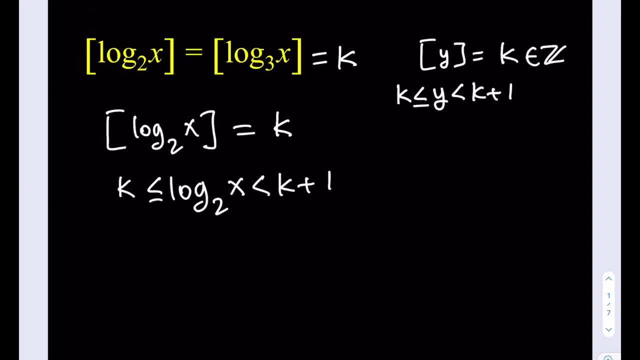 raise everything: 2 to the power, So that's going to look like: 2 to the power k is less than or equal to 2 to the power, log 2x less than 2 to the power k plus 1.. Now what is that supposed to mean? Well, 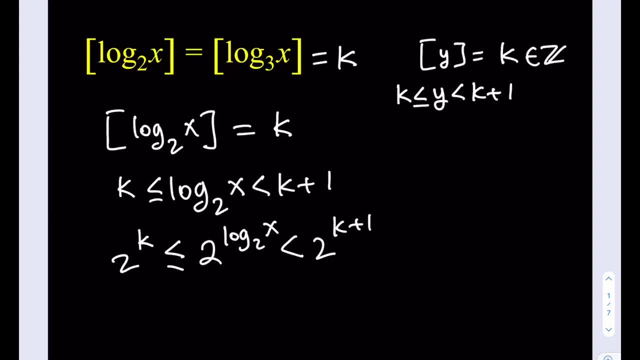 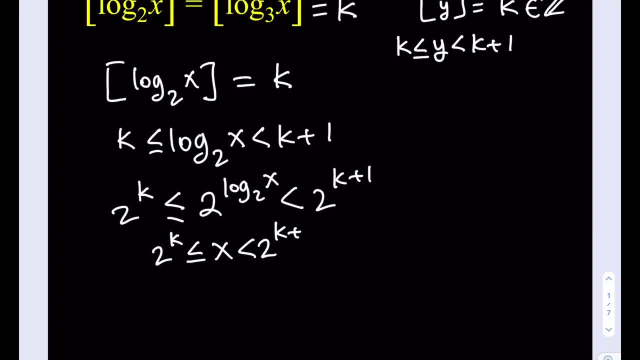 it just means that this is equal to x in the middle, So we can just take the x from there. x is between 2 to the power k and 2 to the power k plus 1, where k is an integer. okay, so that's basically part of our. 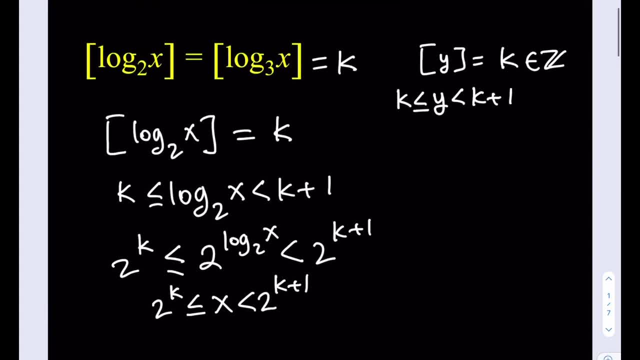 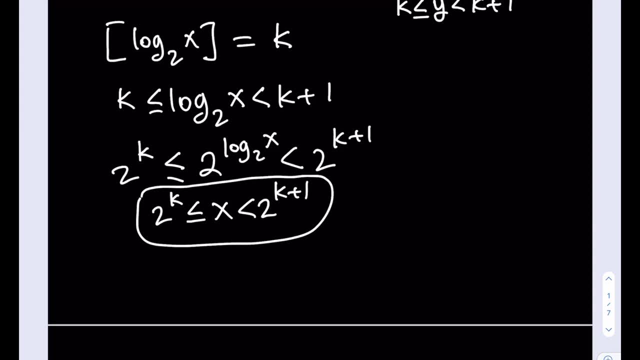 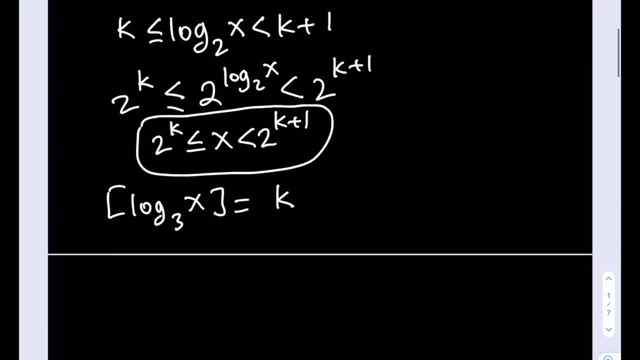 equation. now, let's go ahead and do the same thing for base 3. so let's see what we get from there. so that's one of the inequalities that i'm getting from here. so equation turning into an inequality. basically, okay, let's do the same thing with base 3. so if this is equal to k, then i can safely say: 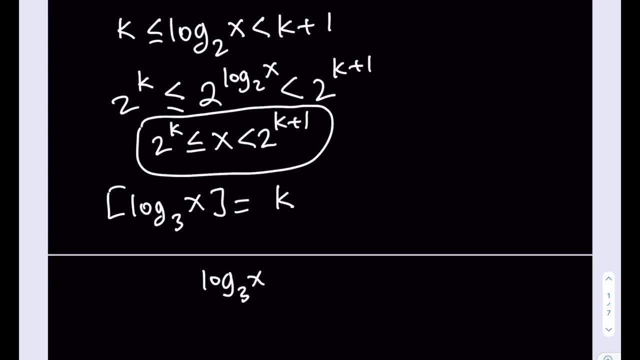 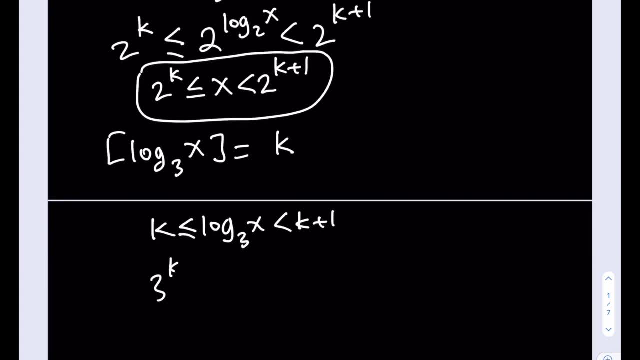 that log 3x is going to be between k and k plus 1, which means 3 to the power. k is less than or equal to 3 to the power. log x with base 3 less than 3 to the power k plus 1, as you know by. 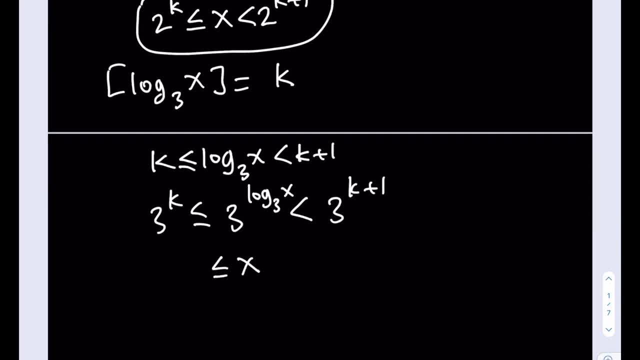 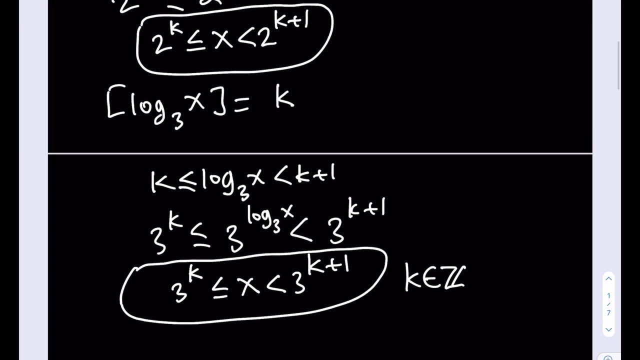 definition, this is going to equal x. so x is going to be between 3 to the power k and 3 to the power k plus 1, where k is an integer like before. so you, this is my second inequality. okay, awesome, now i have two inequalities and i need to solve for x. 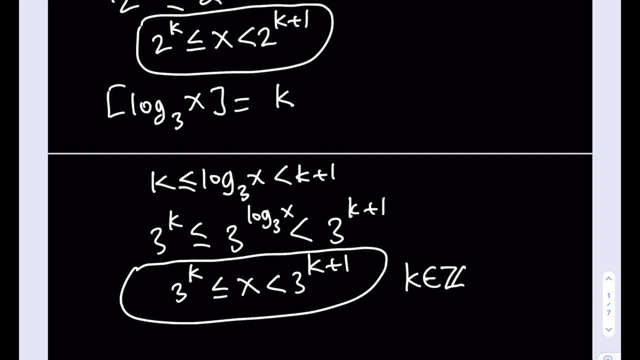 so we just use k as a substitution formula. so how do we solve for x from here? well, we have to consider several different values of k. k is an integer, so k can k be anything. so is it possible for k to be a real large or is it real small? so we're going to test some values here, so why don't? 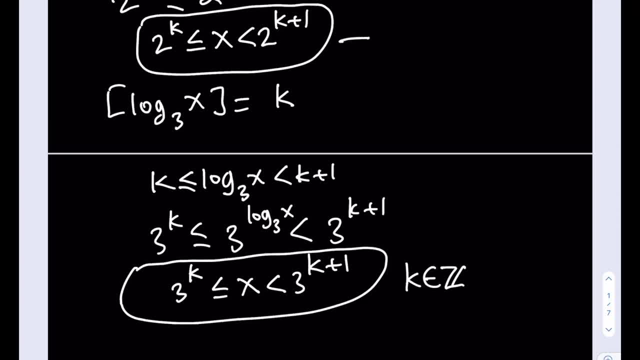 we start with k equals zero, for example. what was if k is equal to zero? so let's go ahead and check it out. if k is equal to zero, then i'm going to be getting x between one and two to the power one, which is two, and from here, if k is equal to. 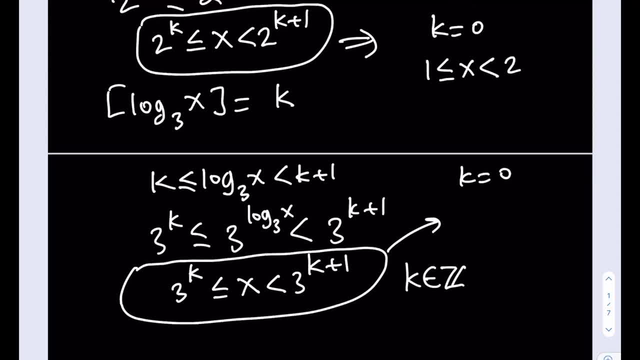 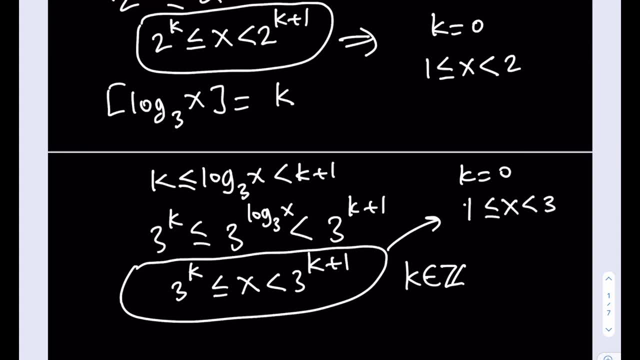 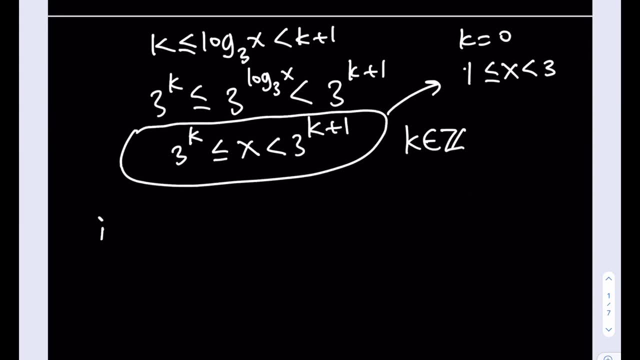 zero, then i'll be getting x between. if k equals zero, then it's going to be one as well. right between one and three. so what? what is that supposed to mean? let's go ahead and write this in a more systematic way. so if k is equal to zero, then x is between one and two. 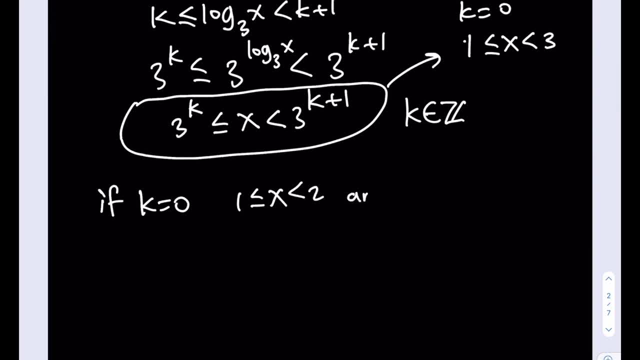 and it's between one and three. obviously, the lower numbers are always included. okay, when you think about this, both of them need to be satisfied. so we're going to look at the intersection. what is that supposed to mean? it means if k is equal to zero, x needs to be between one and two. 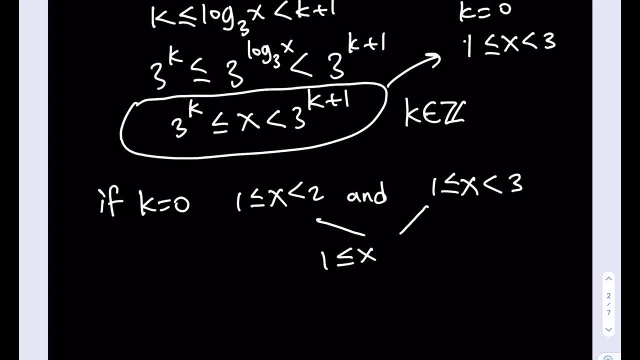 because the intersection of these two inequalities is just going to get bigger and bigger and bigger. so if k is equal to zero, then it's going to give us the interval one and two. okay, we can also write this in the interval notation as using the brackets and parentheses, like this: okay, so that's. 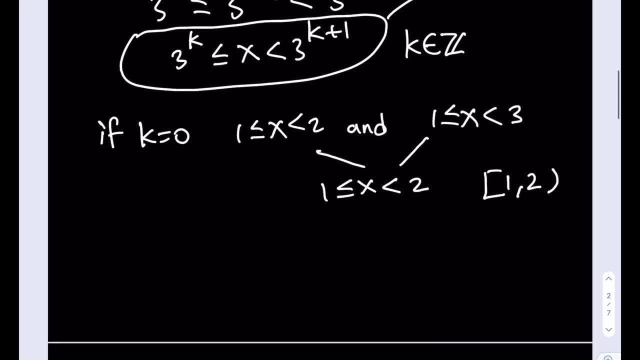 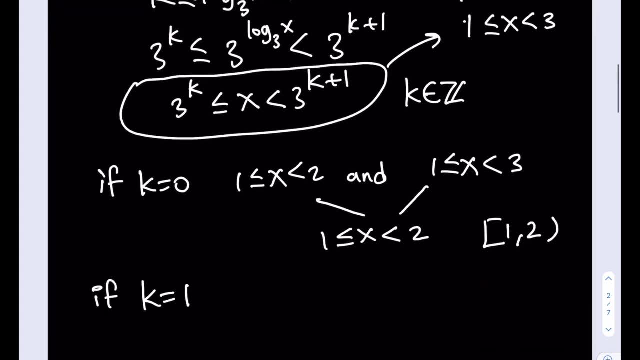 going to be part of our solution. are there other solutions we have to check? so let's go ahead and check it for k equals one. now if k equals one- and you're going to need to refer back to this, but basically it's the same inequality, except the base is two. so let's go ahead and write it down from. 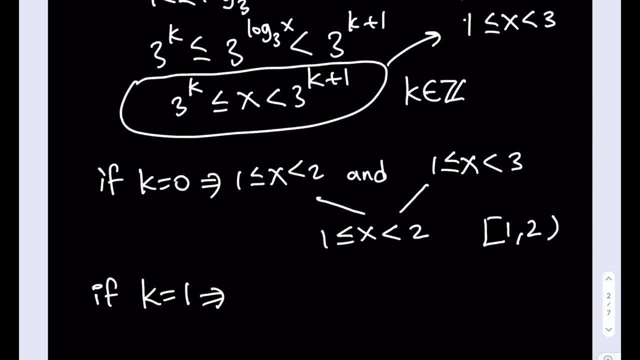 here: if k is equal to zero, then it's going to give us the interval one and two. okay, we can also write it down from here: if k is equal to one, then x is going to be between two to the power one, which is two, and two to the power two, which is four, and basically those are consecutive powers of two and. 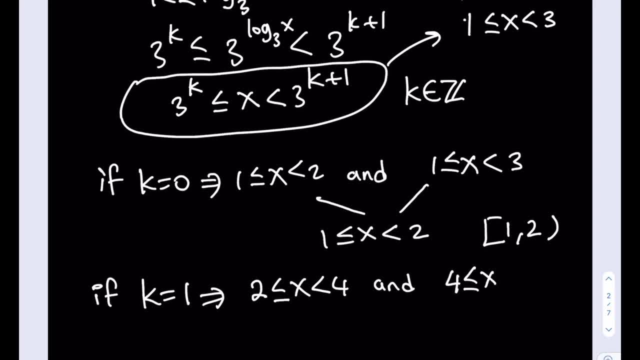 we just pick up where one of them left, and that's going to be between four and eight. now, if you think about these two inequalities, they overlap right. so where do they overlap? well, actually, if they don't right, there's no overlap. so actually we made a mistake here. let's go ahead and do it. 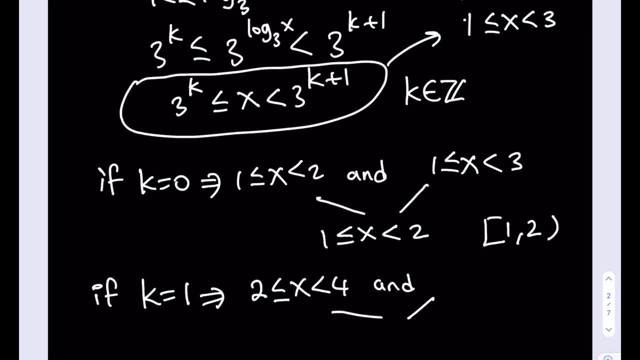 fix that. that's not right. okay, we have to do it for three. so if k is equal to one, then x is going to be between three to the power one, which is three in this case, and the other one is going to be nine. i'm like they don't intersect, they should, okay, so between two and four, and three and nine. 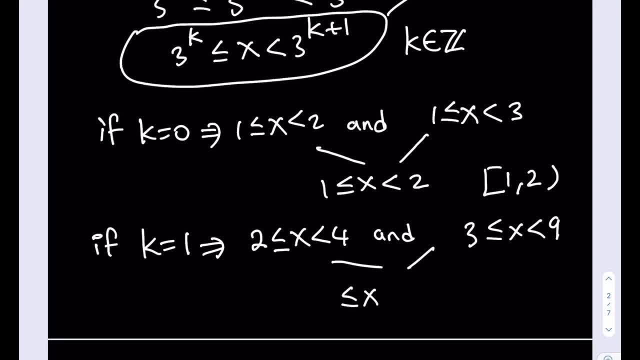 so, if you think about it, then your intersection is going to include the three and not the four. right, because four is not included. it's not going to be in the intersection, so you can write this as interval like this one. okay, again, this is another piece. we're just going to continue. is this going? 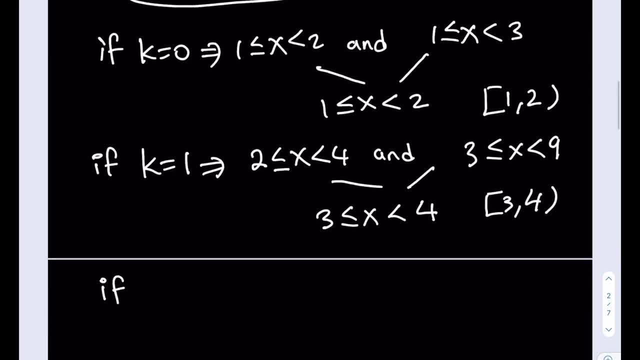 to continue forever. we'll find out. okay, let's see what happens. if k is equal to two, then we're going to be getting x between four and eight and x between nine and twenty seven. so we're just going to go to the cubes, right, because we have k plus one here and that's going to give us the third. 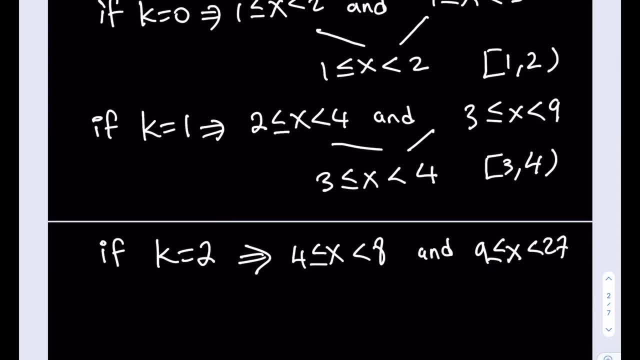 powers. okay, cool, now think about it and if it doesn't make sense, just draw a number line. so i have the four, i have the eight. doesn't have to be drawn to, scale, doesn't really matter. okay, so four is included, eight is not. that's an. 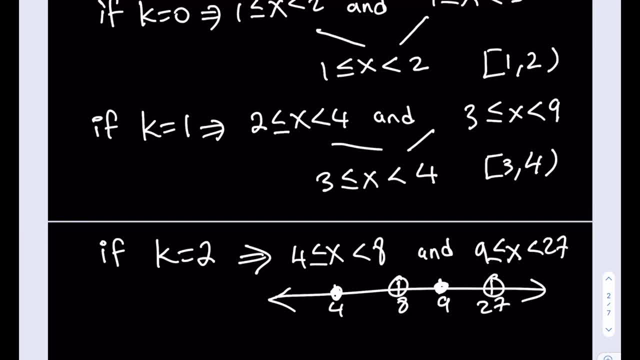 open dot, closed dot and an open dot. so one of my intervals is this one and the other interval is this one, so they are not connected, they don't overlap, so there is no intersection. the solution here is actually empty set. so part of my solution is empty set. what happens if i union that to the other one? nothing, okay, it's kind of. 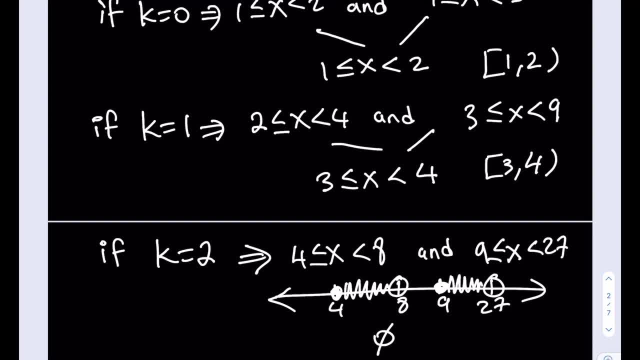 like adding zero. so far i have those two pieces. are there other pieces? well, you notice that as soon as the numbers start getting larger- like k equals two, the second powers, third powers, they're more and more apart. so now at the third power, this difference is going to be bigger. so 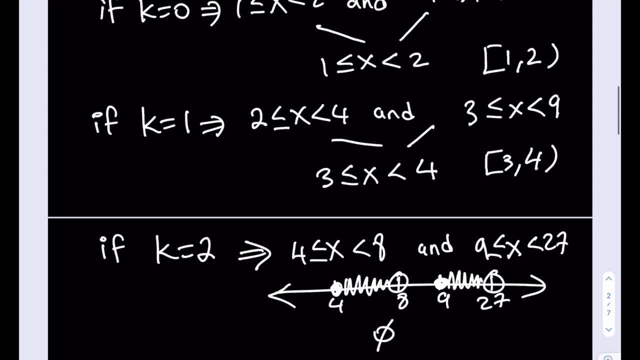 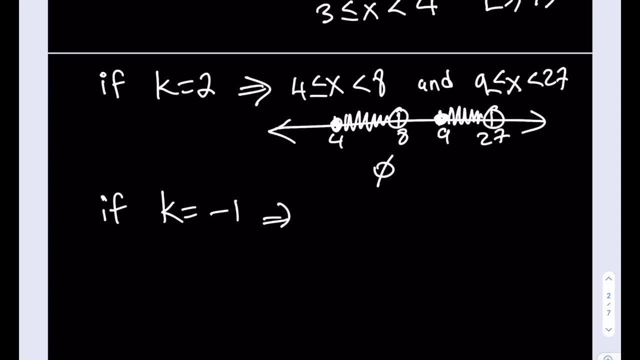 they'll never meet again. okay, so we're done with the positives. let's go ahead and check the negative numbers. what about the negatives? is that going to be a similar pattern? let's find out. if k is equal to negative one, then i'm supposed to have two to the power, negative one. 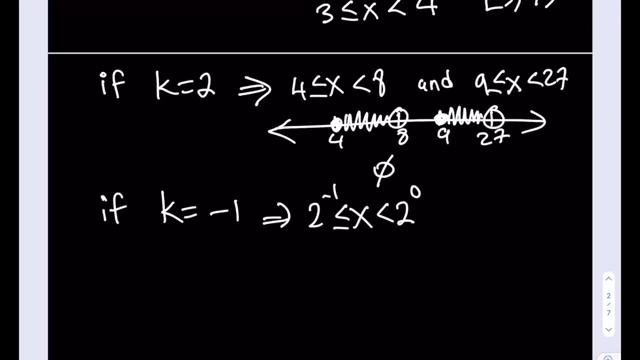 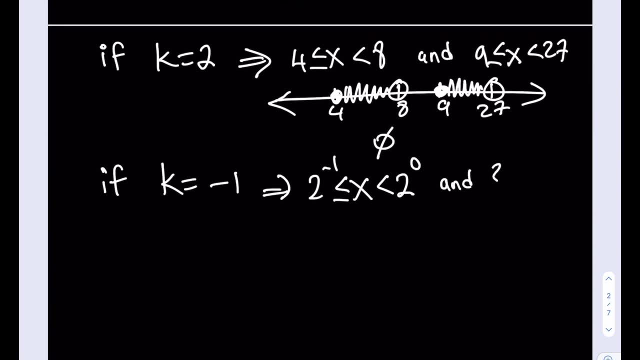 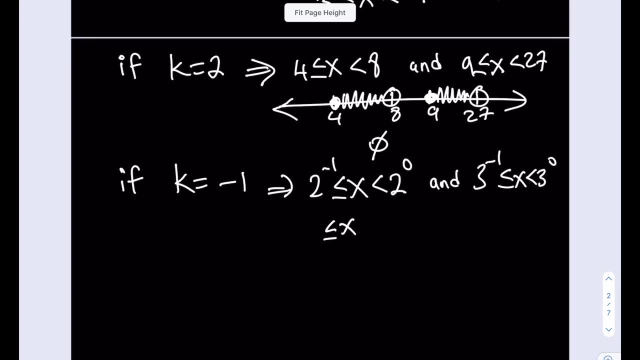 here and two to the power. zero here, right, because we have k and k plus one, so it's going to be negative. one and zero, and the same thing goes for three and it's going to be very, very similar. okay, what is that supposed to mean? this means that x is between one half and one and x is between one. 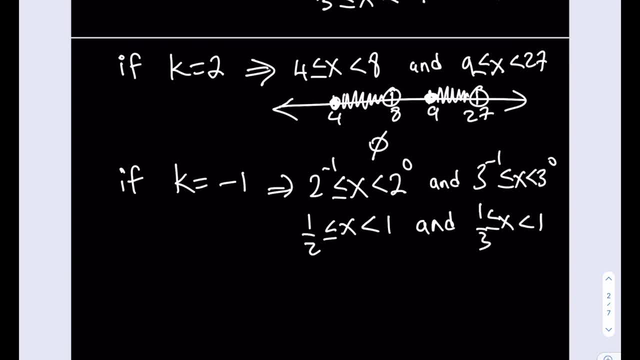 third and one. okay, do you think there's an intersection? yes, because well, they're both between something and one, so they're definitely going to intersect somewhere. but what is that intersection? well, since one third is smaller than one half, their intersection is going to be between one half and 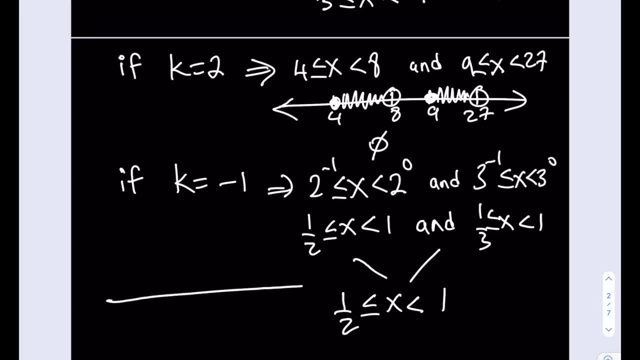 one. you can also verify that by drawing a number line, putting the numbers here: one third, one half and one. one of them is going to be this one and the other interval is going to be this one. their intersection is definitely going to include one half and, but not one. okay, so this is another. 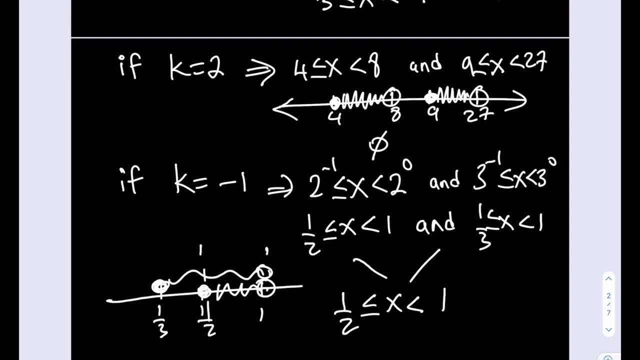 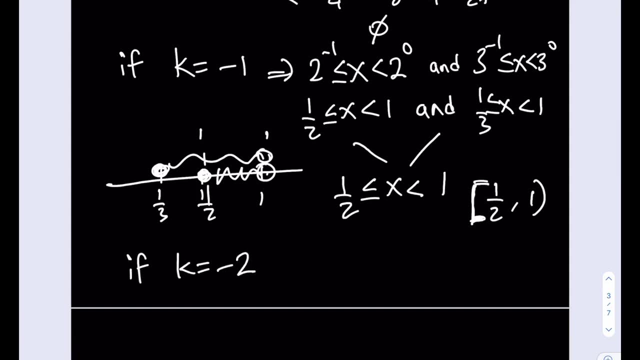 interval that we can kind of piece together with the other ones again with the half closed pattern, one half to one. okay, all right, so let's check out. negative two. do you think there's going to be a solution? let's check it out. okay, if k is negative two, then we got two to the power. negative. 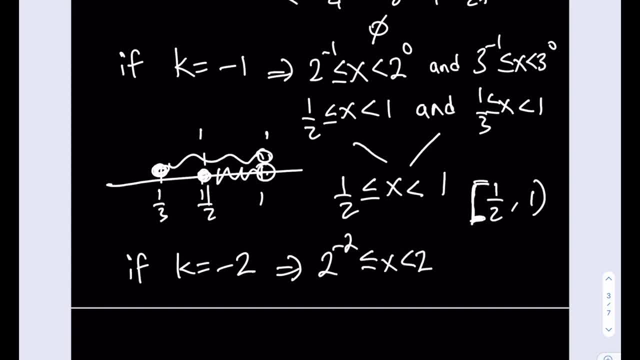 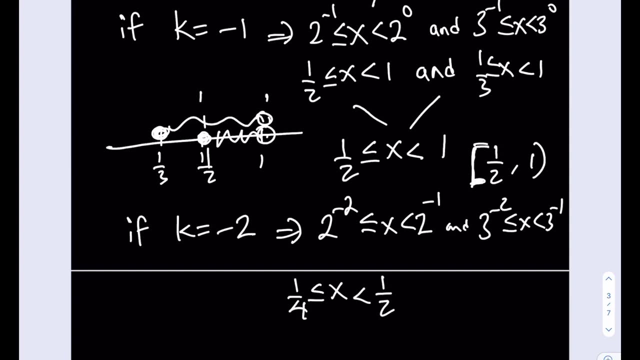 two x and two to the power negative one, and we get three to the power negative two with three to the power negative one, which means x is between one fourth and one half and at the same time, it needs to be between one ninth and one third. okay, what do you think about this? do you think one third is between: 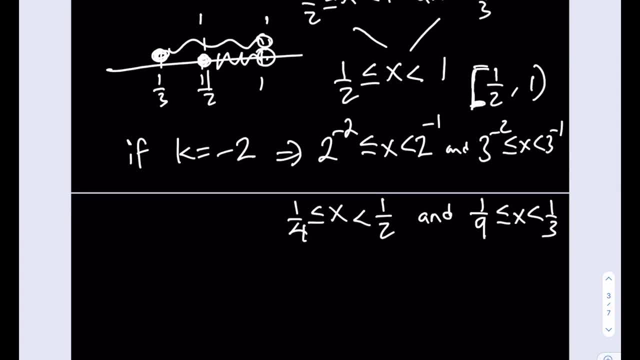 one half and one fourth. yes, but one third is not included. one ninth is definitely not included, and so we have to figure out how to do this. so we have to figure out how to do this. so we have to figure out how to do this. okay, so car doesn't rank in one fourth now. 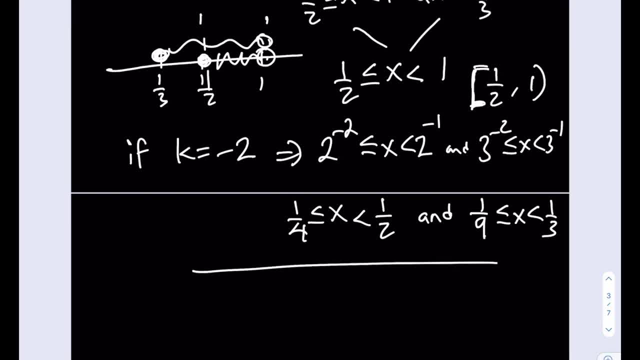 because 1and 2 are definitely way smaller than one fourth. so what's going to happen? okay, let's draw a number line and see what happens. one ninth is the smallest number, and then I have the one fourth, and then I have the one third and then the one half. okay, so the intersection of these two. 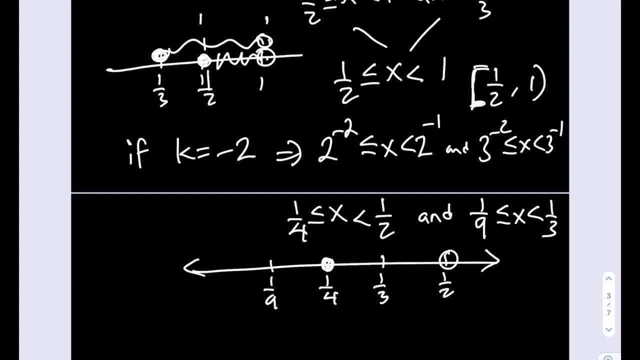 inequalities is going to be what. so I have one of them is going to look like this, right, and the other one is going to be this one and this one, so it's going to look like this. obviously there's an intersection. the intersection is between one fourth and one fourth. the intersection is colors. 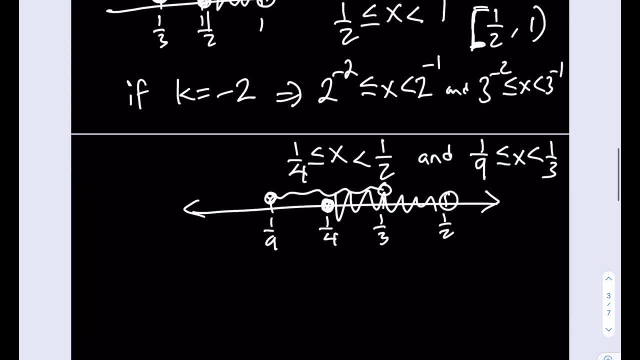 one-third and one-fourth is included- awesome. so then our solution is going to be between one-third- i mean one-fourth and one-third, but one-third is not included because it's not included in one of the inequalities. it needs to be both okay, and, as you know, we can write this in the interval notation. 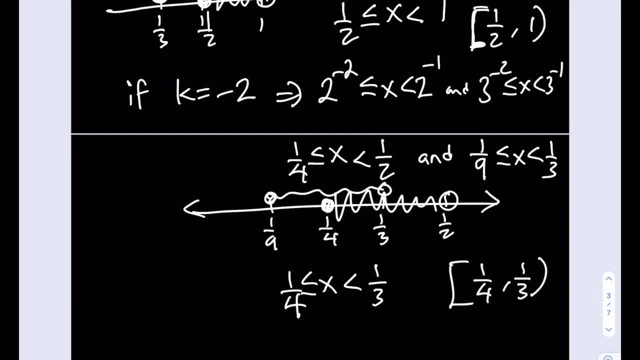 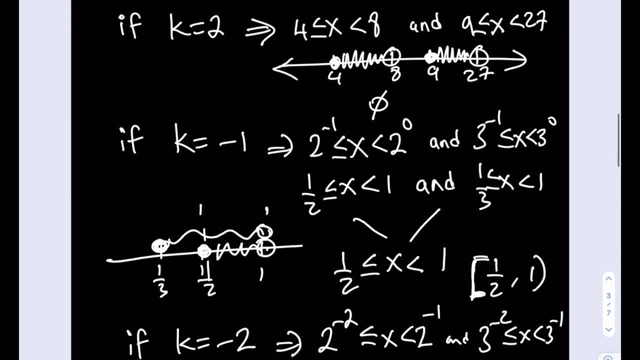 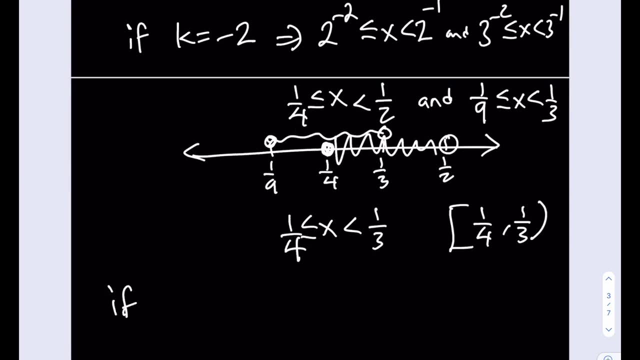 again with one-fourth and one-third like this: awesome. so we got so far how many pieces? one, two, three and four pieces. okay, so let's go ahead and take a look at. k equals negative three. what happens at k equals negative three. that's going to be interesting, okay. so now we're getting two. 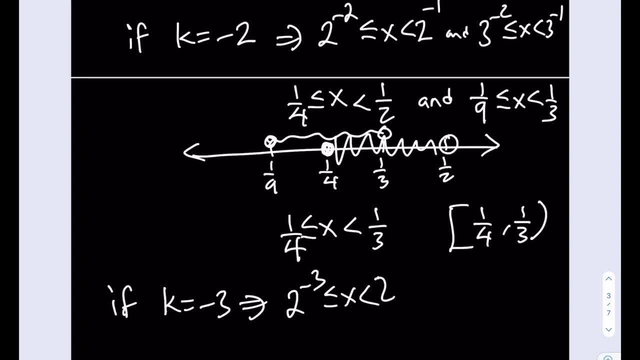 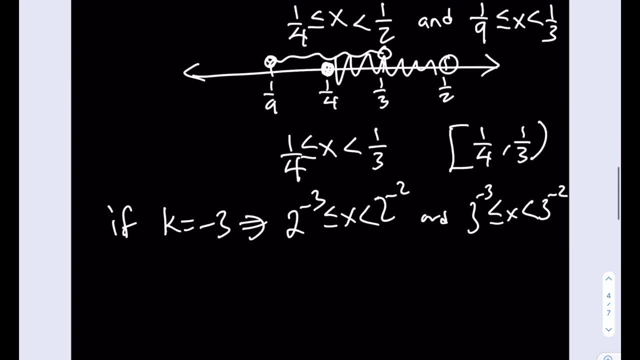 to power negative three with two to power negative two and three to the power negative three with three to the power negative two, and that's going to turn into what? one-eighth and one-fourth, and one over 27 with one over nine- awesome, okay, what happens here? again, we can do our number line to see what. 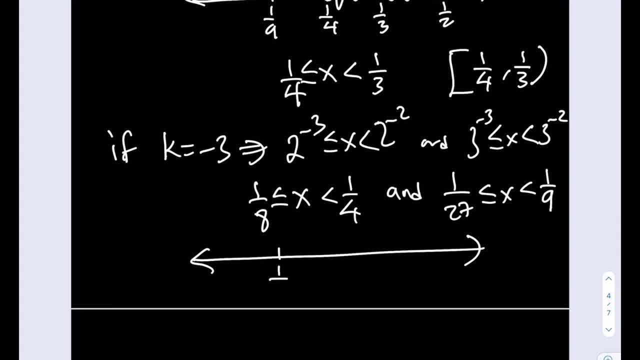 happens, or maybe you already figured it out. smallest number is one over 27 and then one over nine, and then one over eight and then one over four. okay, awesome. the first inequality tells us you're going to be between these two numbers. the second inequality says you've got to be between: 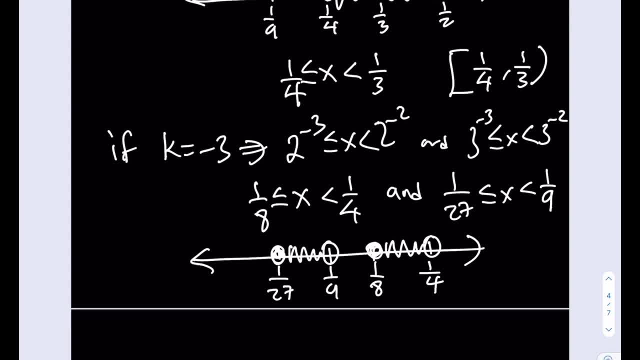 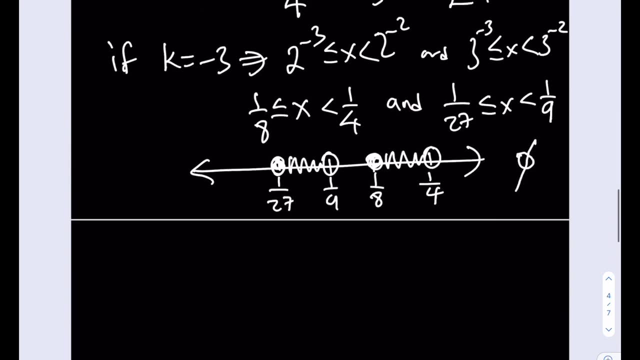 these two numbers, and obviously one-ninth is less than one-eighth. they don't overlap, there's no intersection, there's no solution from here. so the solution set is empty set. so far, we have the following pieces then: right, we have one, two, three, four. let's go ahead and write them down. we have one, two, three, four and we should have a total of: